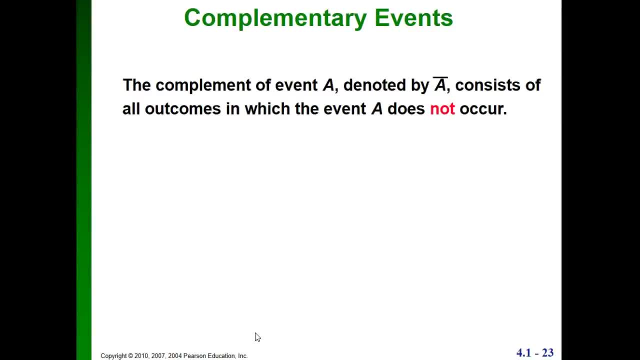 Let's talk about probabilities where they have to do with complementary events. So the complement of an event A, which in this book is denoted by A with a line over the top, consists of all outcomes in which the event A does not occur. 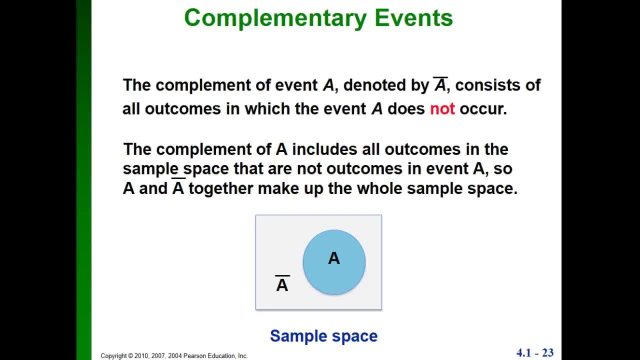 So the complement of A includes all the outcomes in the sample space that are not outcomes in the event A. That means A and A complement together make up the whole sample space. Here we have a picture. This is the whole sample space inside of this box. 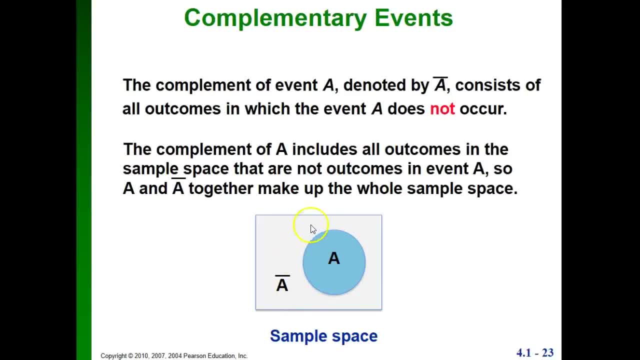 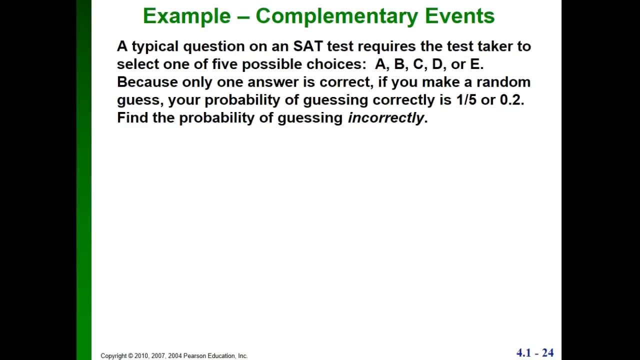 This in the circle is the event A. so everything outside of the circle is the complement of A. So if we put those two together, A and A complement, they give us the whole sample space. An example of complementary events It is that 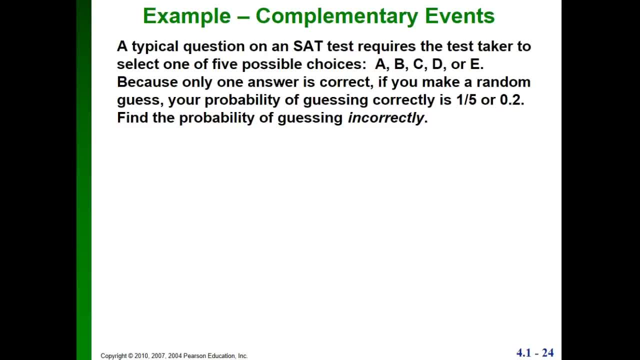 A typical question on an SAT test requires the test taker to select one of five possible choices- A, B, C, D or E- Because only one answer is correct. if you make a random guess, your probability of guessing correctly is 1 fifth or 0.2. 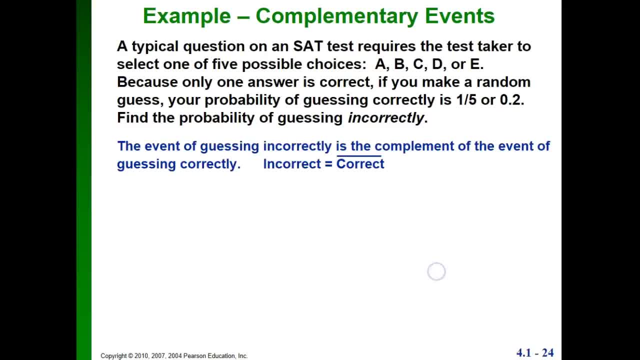 If we want to find the probability of guessing incorrectly. guessing incorrectly is the complement of the event of guessing correctly, So incorrect is the complement of correct. Now, exactly one of the five choices is correct. That means that four of the choices are incorrect. 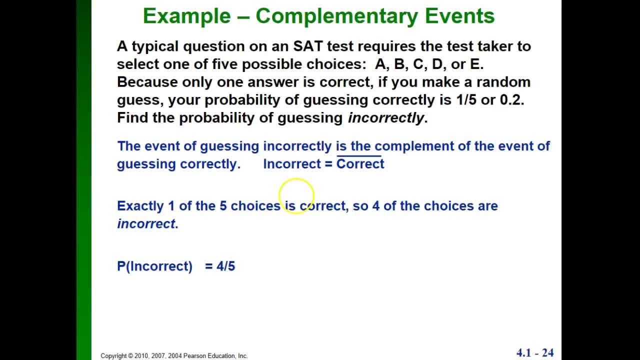 So the probability of guessing incorrectly is 4 over 5, because we had four incorrect choices out of the five total. That means the probability of guessing incorrectly is 4 fifths. Or, if we think about probabilities of complementary events, the answer isều. 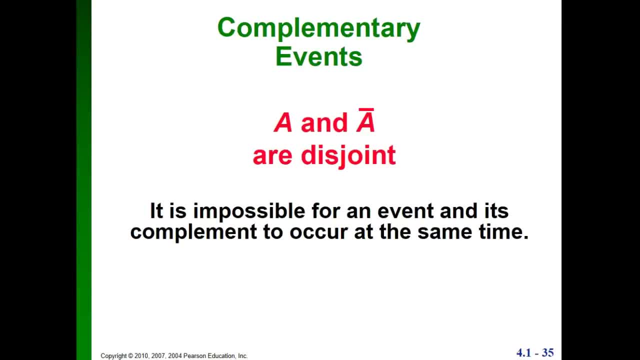 3 fifths, while the probability of guessing incorrectly is 8 fifths and прир petits are not congruence. So Thing A is safe, So Thing B is safe. Now let's take a look atrz key. If we think about probability of RM0, it must be probability of adding a complement to. 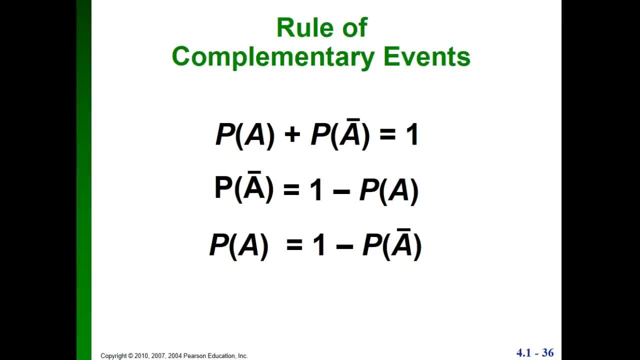 A into the scale of a� compared to level A in a smaller car. Let's see a little longer form for that. If A and A complement are disjoint and if together they make up the whole sample space, then the two probabilities added together should equal 1, because we've got 100% of the 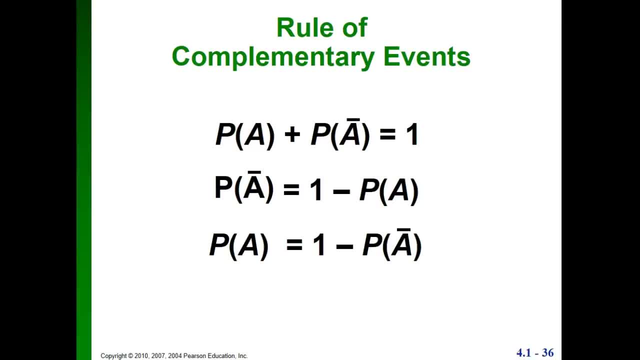 outcomes in the sample space if we put the two events together. So our first rule is that the probability of A plus the probability of A complement is equal to 1. From that we can get two other rules, and this is usually how we use this rule. 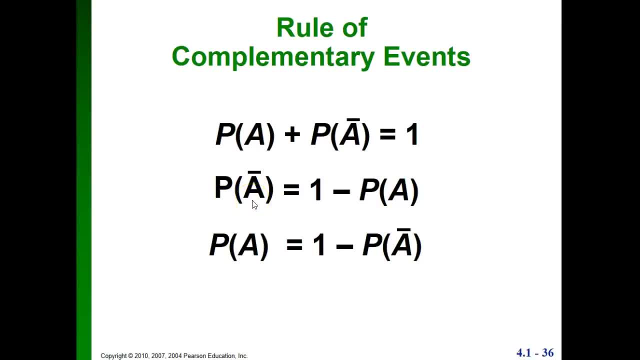 So if we're trying to find the probability of A complement, we can find the probability of A and just subtract it from 1.. Or if we're trying to find the probability of the event A, we can find the probability of its complement and subtract that from 1.. 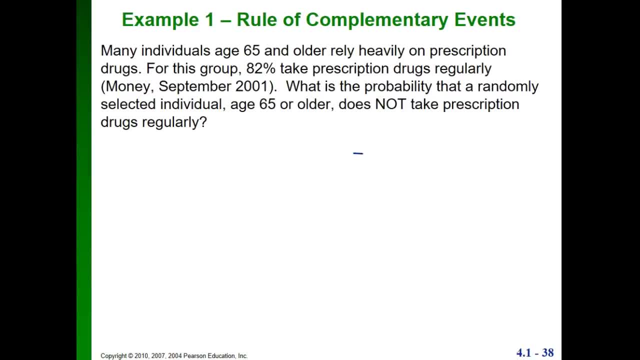 So this rule works either one of those two ways. Let's look at an example of this. Many individuals aged 65 and older rely heavily on prescription drugs. For this group, 82 percent take prescription drugs regularly. This is according to Money Magazine in September 2001.. 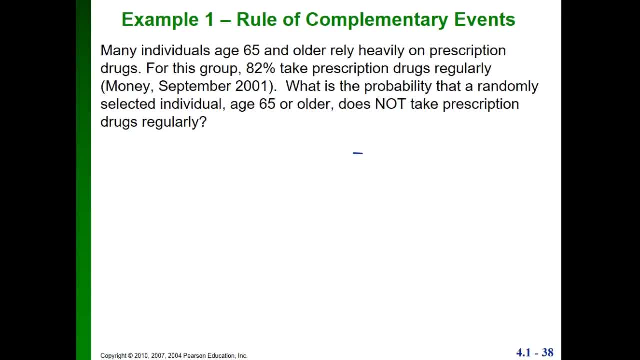 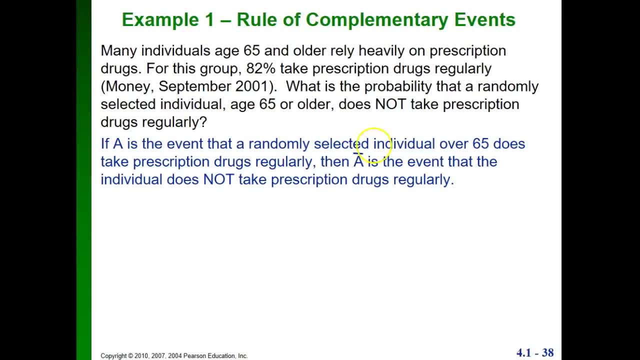 Then A complement, that the individual does not take prescription drugs regularly. now we were told in the information up here that 82% of this group does take these drugs regularly. so that means the probability of event a, which would mean a randomly selected individual does take drugs regularly, would be 82%. if we want to, 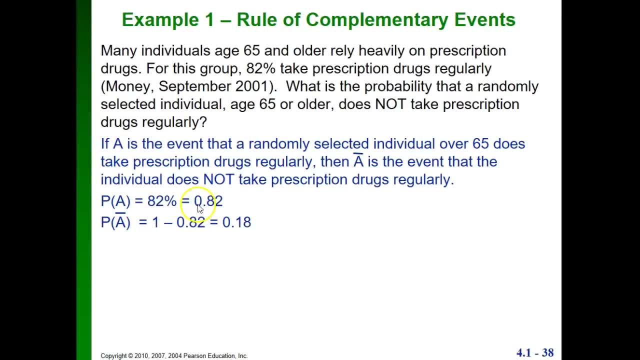 find the probability of the complement, all we have to do is take this value and subtract it from 1. so the probability of a complement would be the probability that the randomly selected individual does not take prescription drugs regularly. that would be 1 minus 0.82, and that would be 0.18 or 18%. here's another. 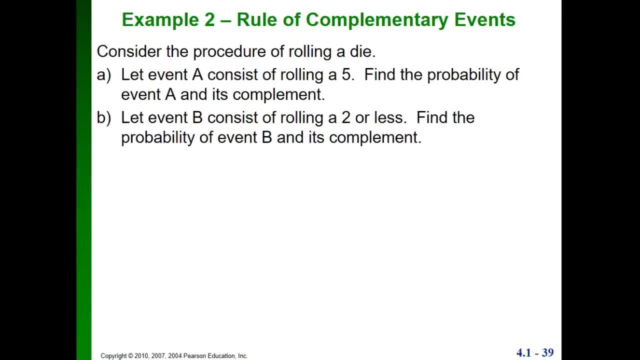 example, if we consider the procedure of rolling the dice, we can see that the individual does not take prescription drugs regularly. let event a consist of rolling a 5, find the probability event, event a and its complement, and then we're going to let event B consist of rolling a 2 or less. 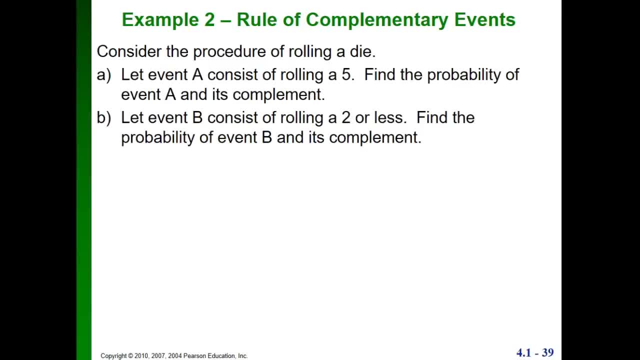 and we're going to find the probability event of event B and its complement. so for part a of this, the event a includes just one outcome and that is that we roll a 5. the complement of a is the event of not rolling a 5, since our sample space is all six faces on the. 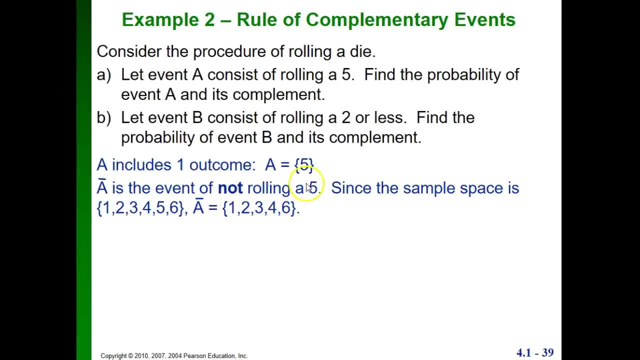 die. that means a complement is every face except for the five, so it's one, two, three, four and six. the probability of a, since there was only one outcome in event a, is one sixth and the probability of a complement is five sixths. so we could get this by either noticing how many 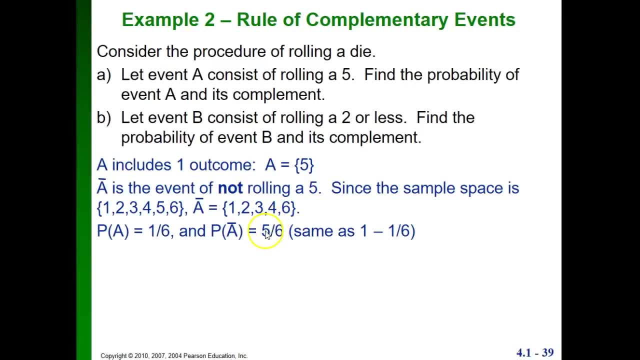 events were in our a complement, which is five, or we could just simply take the probability for a and subtract that from one. either way, we would get 5 sixths. now for part B in this question. the event B consists of rolling a, 2 or less that. 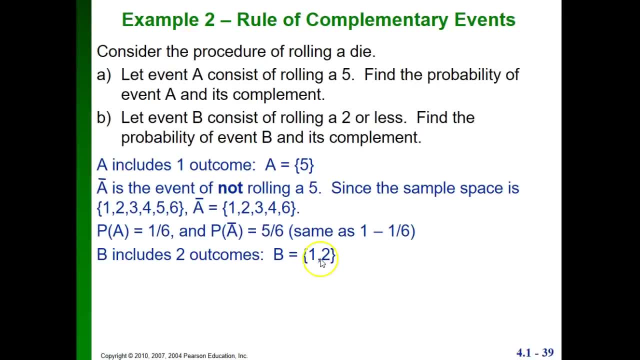 includes two outcomes, because that could either be rolling a one or rolling it. to so be complimented would be every other face on the die that's not already included in this set, which would be three, four, five and six. the probability of b, since there were two simple events in this event, would be two. 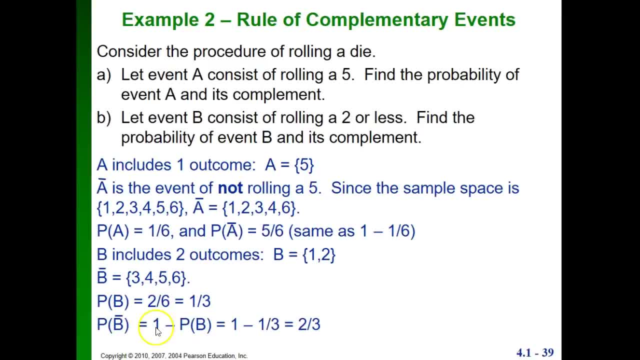 or six, which would simplify to one-third. the probability of b complement would be one minus this. so one minus one-third would equal two-thirds. we could also get that answer by looking at how many simple events are in b complement. therefore, out of the six in the sample space, four-sixths.